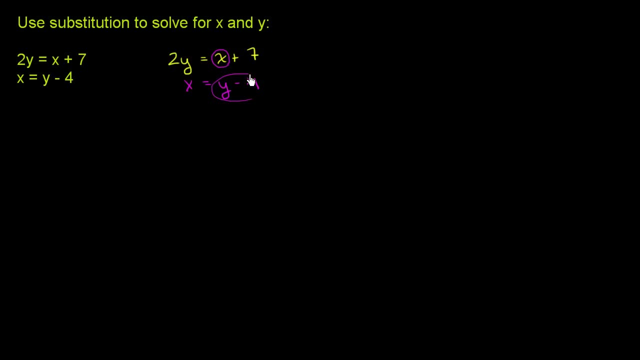 So everywhere we see an x, we can substitute it with a y minus 4.. So let's do that. So if we substitute y minus 4 for x in this top equation, the top equation becomes: 2y is equal to, instead of an x, the. 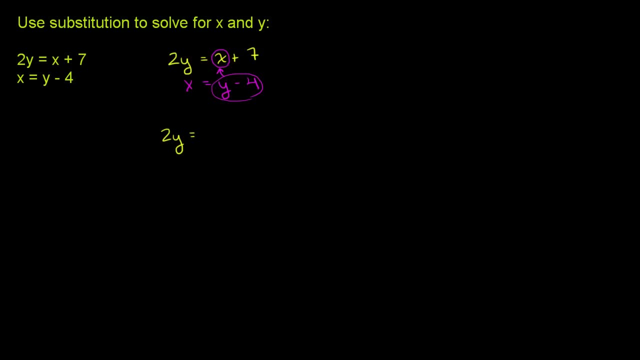 second constraint tells us that x needs to be equal to y minus 4.. So instead of an x, we'll write a y minus 4.. And then we have a plus 7.. All I did here is I substituted. All I did is I substituted y minus 4 for x. 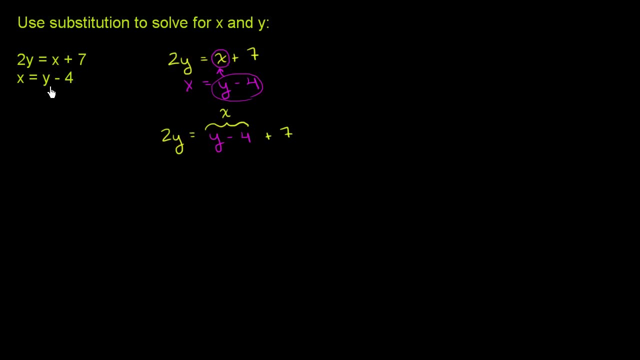 The second constraint tells us that we need to do it. y minus 4 needs to be equal to x, or x needs to be equal to y minus 4.. The value here is. now we have an equation, one equation with one variable. we can just solve for y. 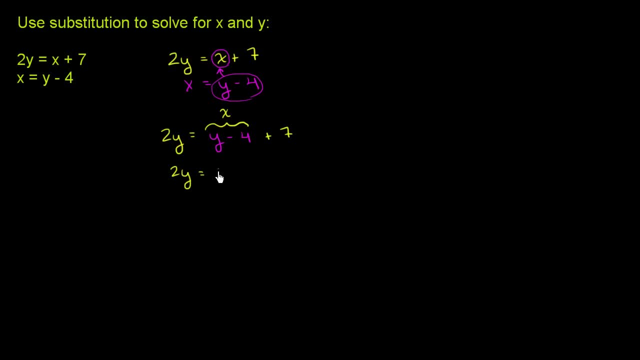 So we get: 2y is equal to y, and then we have minus 4 plus 7. So y plus 3.. We can subtract y from both sides. We can subtract y from both sides. That's good. We can subtract y from both sides of this equation. 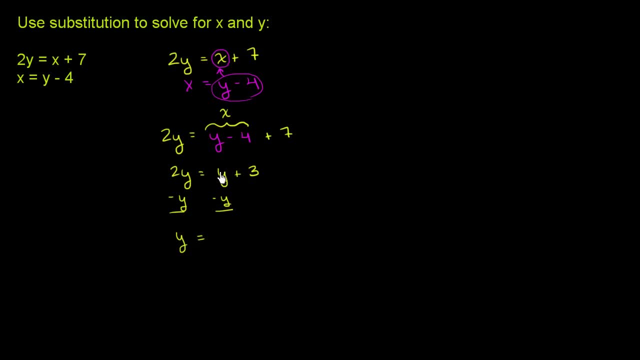 The left-hand side, 2y minus y is just y. y is equal to these. cancel out y is equal to 3.. And then we could go back and substitute into either of these equations to solve for x. This is easier right over here. 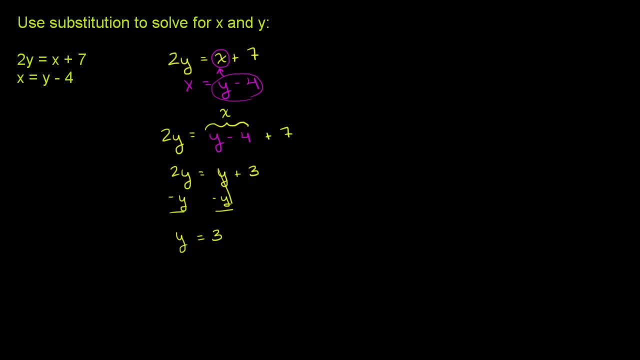 So let's substitute right over here: x needs to be equal to y minus 4.. So we could say that x is equal to 3 minus 4, which is equal to negative 1.. So a solution, the solution to this system is: x is equal to. 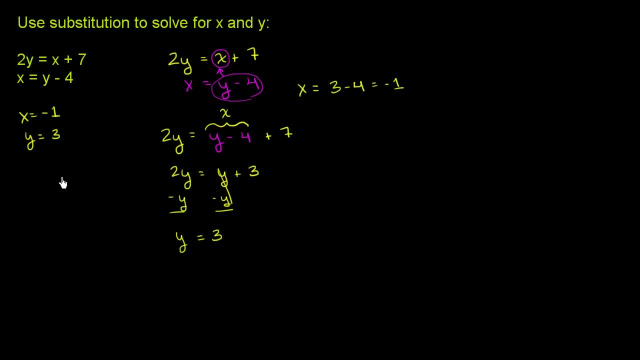 negative 1, and y is equal to 3.. And you can verify that it works in this top equation right over here: 2 times 3 is 6, which is indeed equal to negative 1 plus 7.. Now I want to show you that over here we substituted we. 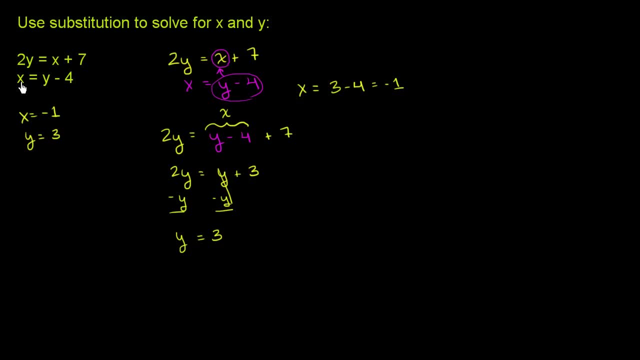 had an equation that explicitly solved for x, So we were able to substitute the x's. What I want to show you is we could have done it the other way around. We could have solved for y And then substituted for the y's. 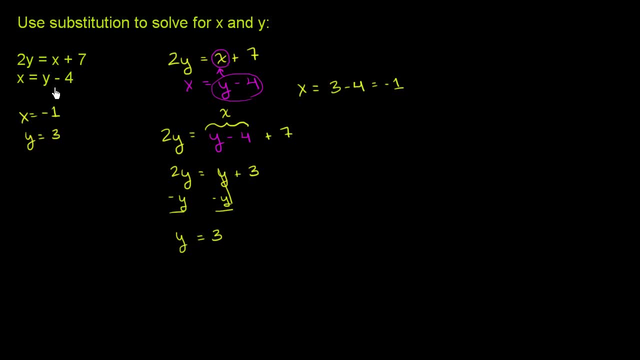 So let's do that, And we could have substituted from one constraint into the other constraint or vice versa. Either way we would have gotten the same exact answer. So instead of saying x is equal to y minus 4, in that second. 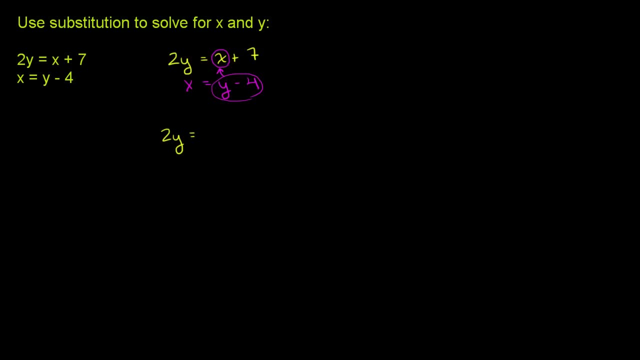 second constraint tells us that x needs to be equal to y minus 4.. So instead of an x, we'll write a y minus 4.. And then we have a plus 7.. All I did here is I substituted. All I did is I substituted y minus 4 for x. 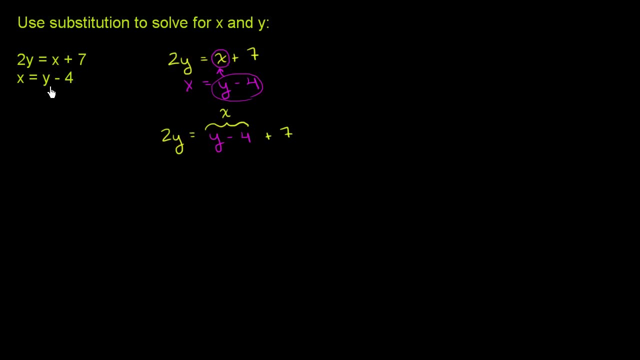 The second constraint tells us that we need to do it. y minus 4 needs to be equal to x, or x needs to be equal to y minus 4.. The value here is. now we have an equation, one equation with one variable. we can just solve for y. 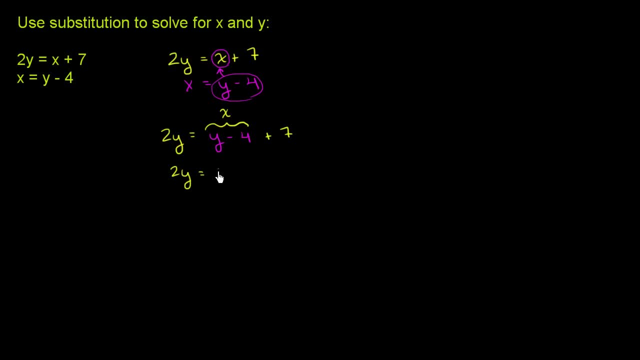 So we get: 2y is equal to y, and then we have minus 4 plus 7. So y plus 3.. We can subtract y from both sides. We can subtract y from both sides. That's good. We can subtract y from both sides of this equation. 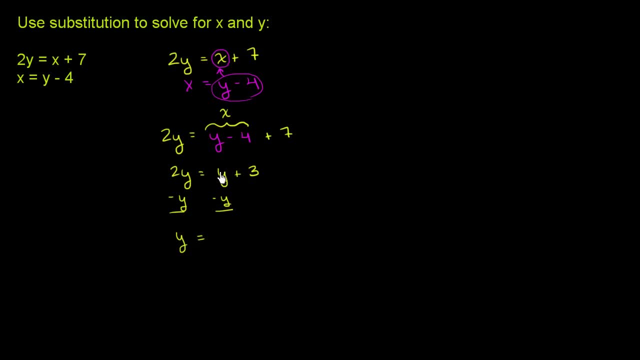 The left-hand side, 2y minus y is just y. y is equal to these. cancel out y is equal to 3.. And then we could go back and substitute into either of these equations to solve for x. This is easier right over here. 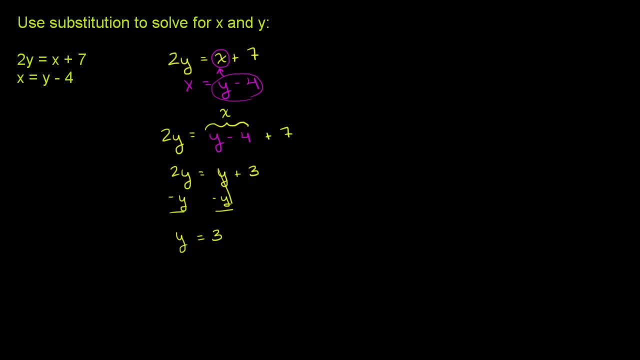 So let's substitute right over here: x needs to be equal to y minus 4.. So we could say that x is equal to 3 minus 4, which is equal to negative 1.. So a solution, the solution to this system is: x is equal to. 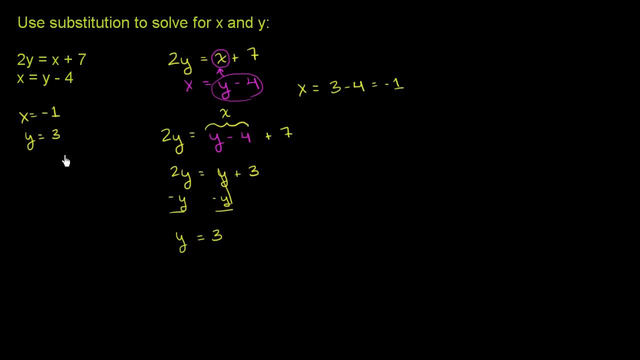 negative 1, and y is equal to 3.. And you can verify that it works in this top equation right over here: 2 times 3 is 6, which is indeed equal to negative 1 plus 7.. Now I want to show you that over here we substituted we. 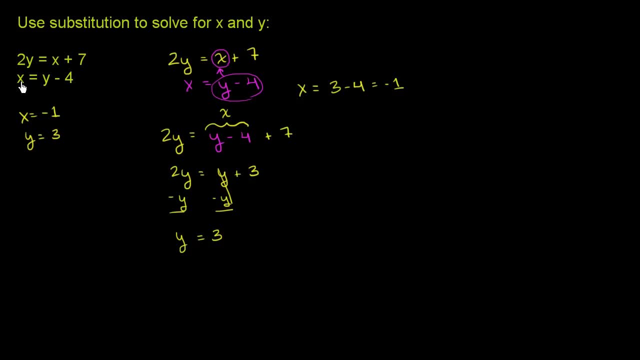 had an equation that explicitly solved for x, So we were able to substitute the x's. What I want to show you is we could have done it the other way around. We could have solved for y And then substituted for the y's. 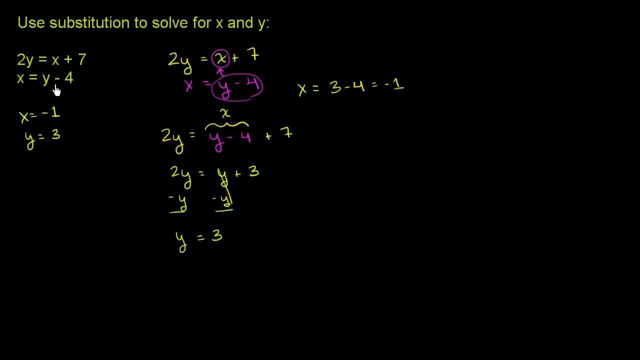 So let's do that, And we could have substituted from one constraint into the other constraint or vice versa. Either way we would have gotten the same exact answer. So instead of saying x is equal to y minus 4, in that second. 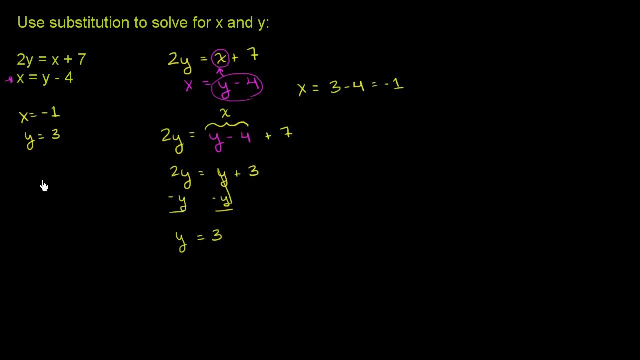 equation. if we add 4 to both sides of this equation, we get x plus 4 is equal to y. This and this is the exact same constraint. I just added 4 to both sides of this to get this constraint over here. 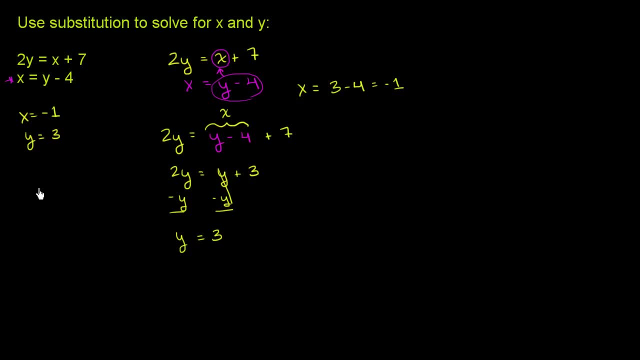 equation. if we add 4 to both sides of this equation, we get x plus 4 is equal to y. This and this is the exact same constraint. I just added 4 to both sides of this to get this constraint over here. 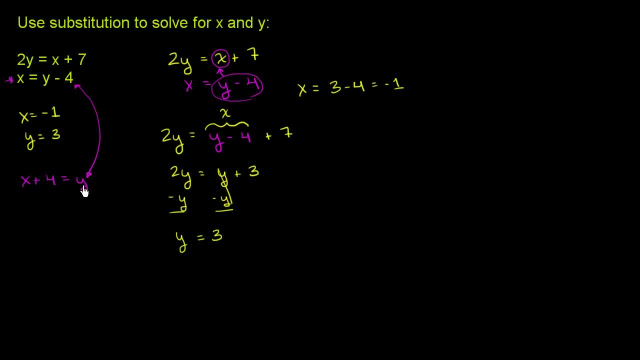 And now, since we've solved for x, we can solve for y. We've solved this equation explicitly for y. We can use the first constraint, the first equation, And everywhere where we see a y, we can substitute it with x plus 4.. 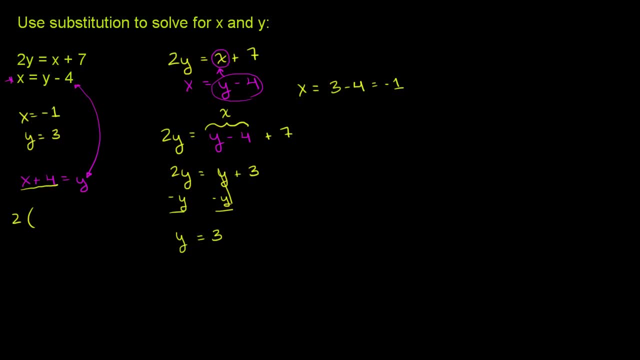 So it's 2 times instead of 2 times y. we can write 2 times x plus 4.. 2 times x plus 4 is equal to x plus 7.. We can distribute this: 2.. So it gets: 2x plus 8 is equal to x plus 7.. 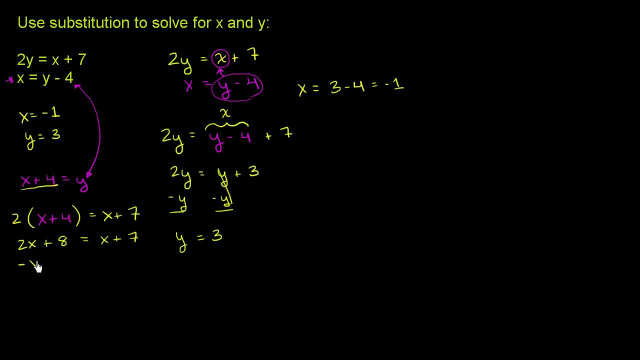 7, we can subtract x from both sides of this equation, and then we can subtract 8 from both sides of this equation: The left-hand side that cancels out. We're just left with an x On the right-hand side that cancels out, and we are left. 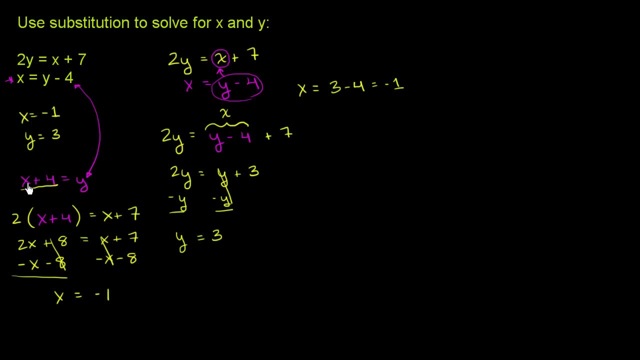 with a negative 1.. Then we can substitute back over here. We have: y is equal to x plus 4.. So y is equal to negative 1 plus 4, which is equal to 3.. So once again we got the same answer, even though this time. 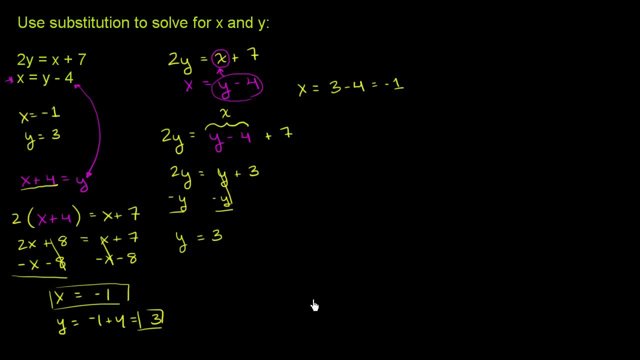 we substituted for y instead of substituting for x. Hopefully you found that interesting. 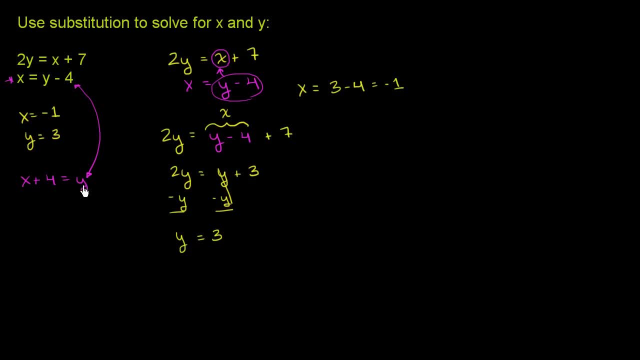 And now, since we've solved for x, we can solve for y. We can solve this equation explicitly for y. we can use the first constraint, the first equation, And everywhere where we see a, y, we can substitute it with x plus 4.. 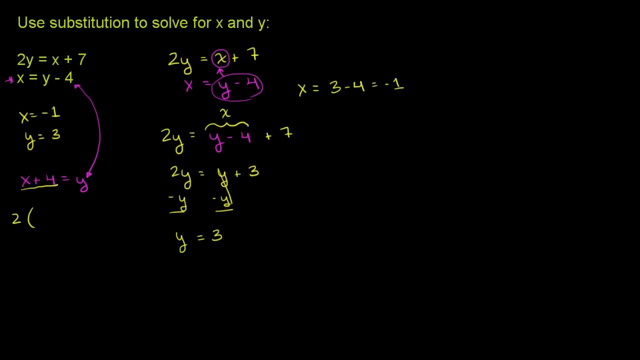 So it's 2 times instead of 2 times y. we can write: 2 times: x plus 4 is equal to x plus 7.. We can distribute this 2,, so it gets: 2x plus 8 is equal to x plus 7.. 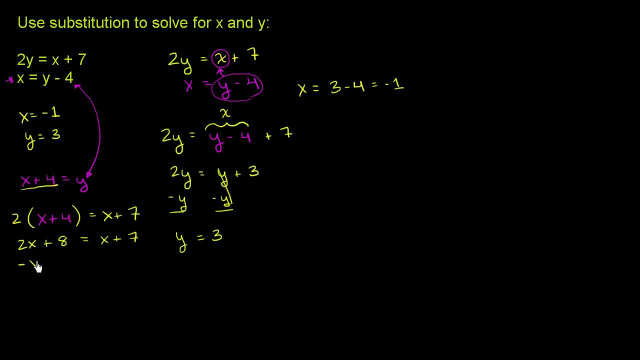 7, we can subtract x from both sides of this equation, and then we can subtract 8 from both sides of this equation: The left-hand side that cancels out. We're just left with an x On the right-hand side that cancels out, and we are left. 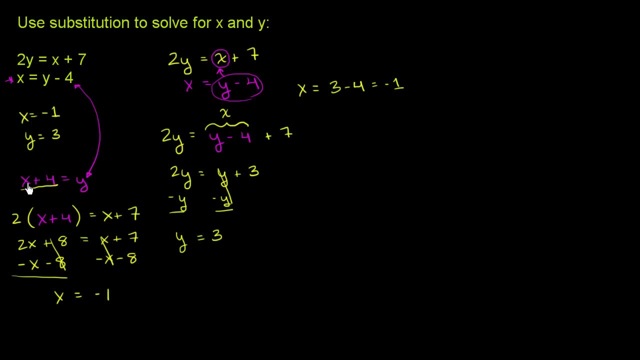 with a negative 1.. Then we can substitute back over here. We have: y is equal to x plus 4.. So y is equal to negative 1 plus 4, which is equal to 3.. So once again we got the same answer, even though this time. 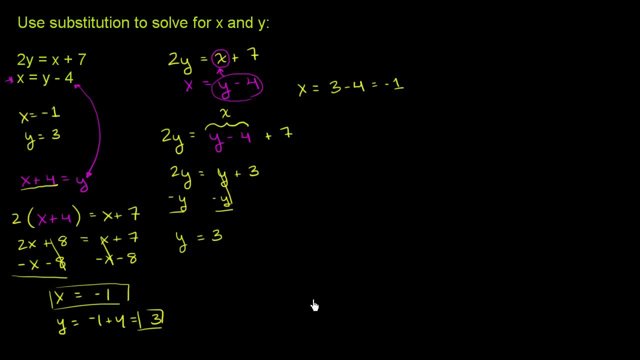 we substituted for y instead of substituting for x. Hopefully you found that interesting.